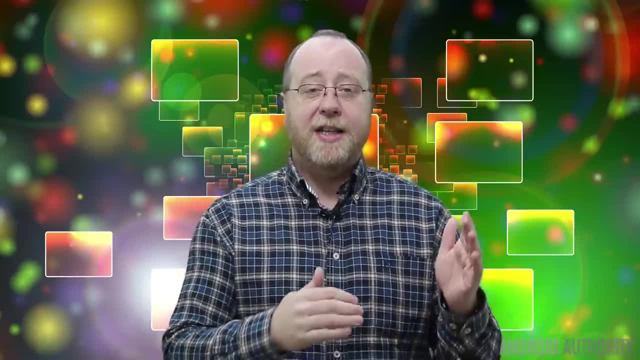 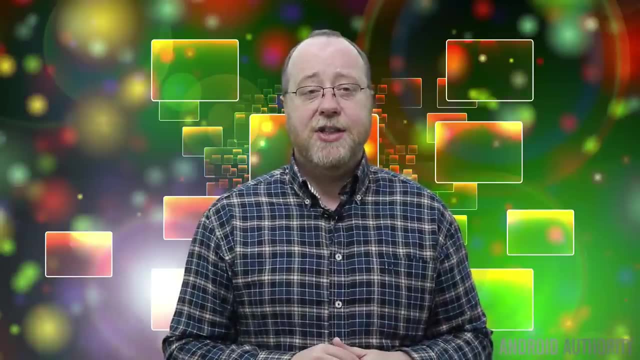 issue of memory fragmentation. If you're trying to run two programs and you allocate one bit of the memory for one program and another bit of memory for another program, and then what happens? The program exits and then you try to write a second one. It might fit in that space of. 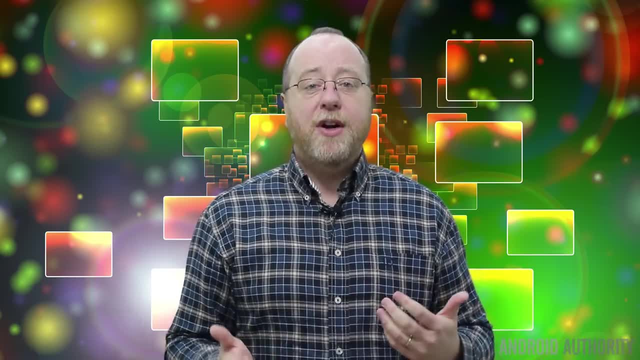 the first app, but maybe it's a bit smaller. So there's a gap left And then when you run a third one, it can't fit in that gap, So it goes somewhere else in memory And then you actually get these little gaps starting to appear And so you get this thing called. 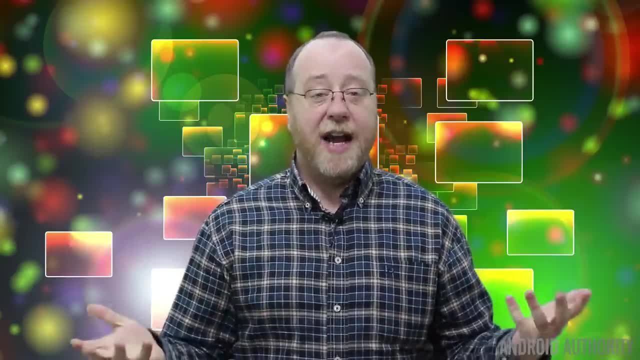 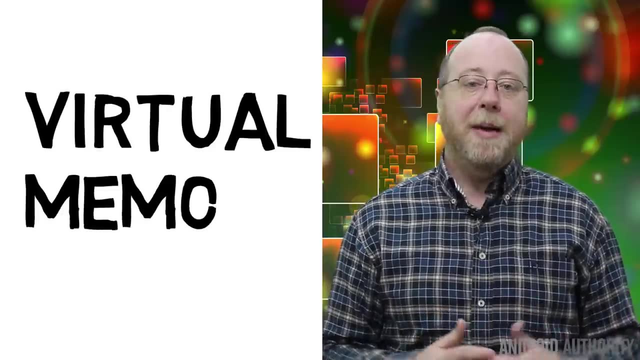 memory fragmentation, And that's a real problem. Eventually you'll run out of memory just because of fragmentation. So to get around these problems we have this technology called virtual memory, And in virtual memory each app that's running on a 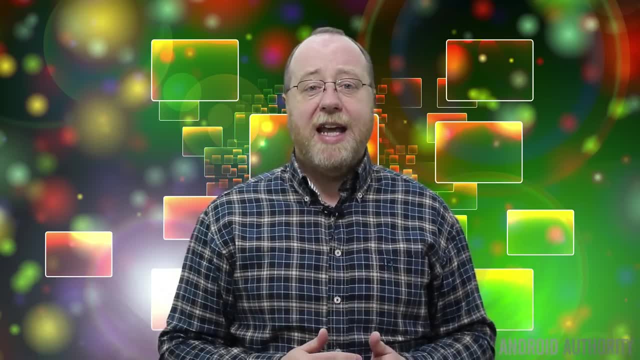 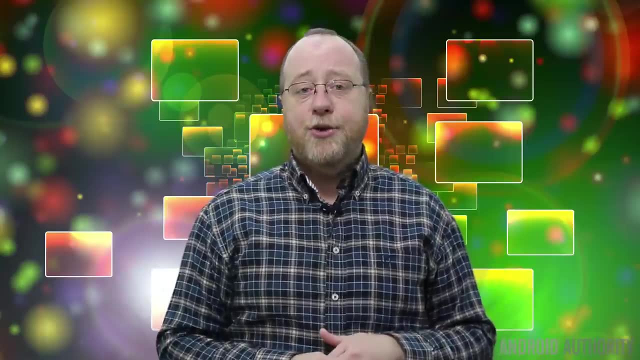 on a mobile phone, each program that's running on Windows or on OS X thinks it's the only app running. It thinks it's the only program running And it has access to all of the address space. In fact, it doesn't even have to have that amount of physical memory On a 32-bit. 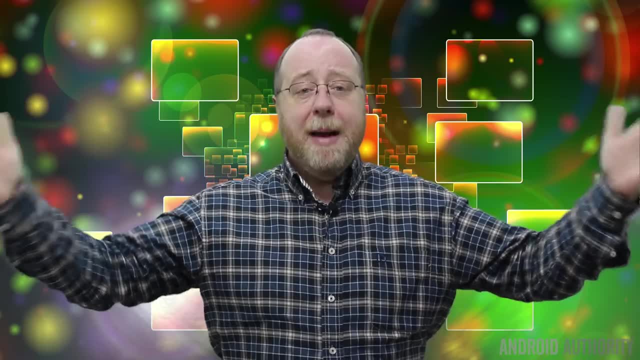 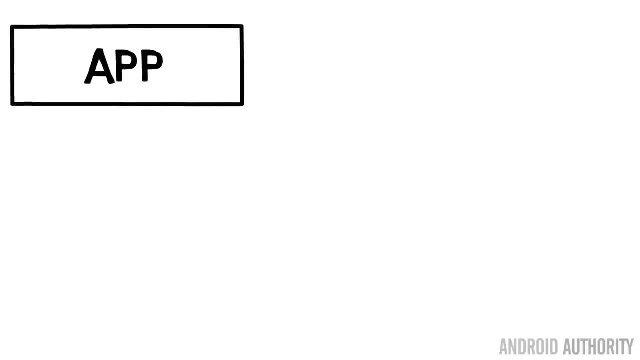 machine. that process thinks it has 32 bits worth of memory to play with, which is, of course, four gigabytes, And the way it works is this: When the process, when the app wants to access a particular address, it's going to have to have a certain amount of memory. 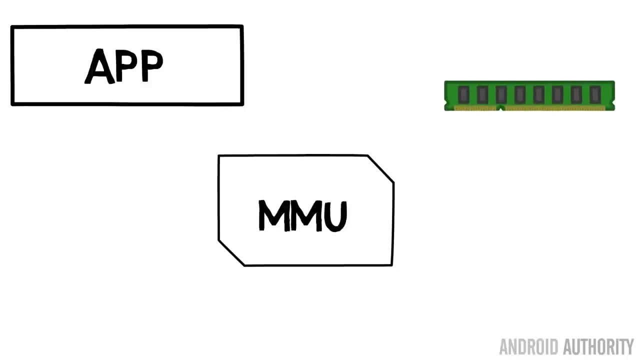 It's going to have to have a certain amount of memory. It's going to have to have a certain amount of memory. There is a particular piece of hardware in the CPU called the MMU, the memory management unit, And what it does is it maps from this virtual address that. 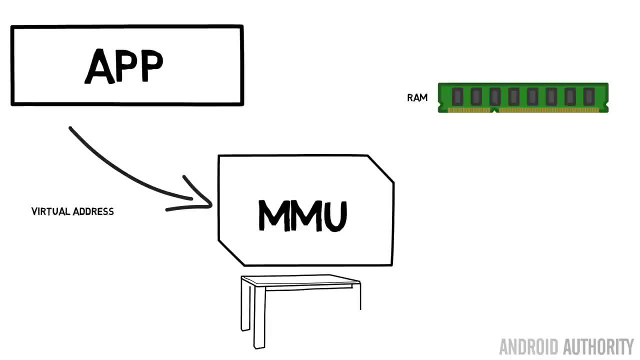 the app thinks it's running in to an actual physical address somewhere in memory, And so now the idea of partitioning up the memory is actually taken over by the operating system and the app doesn't need to worry. The app thinks it's the only app running It can write. 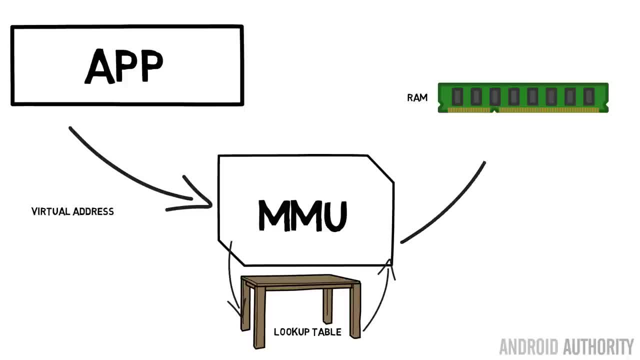 to whatever addresses it's allowed to, whichever memory it's been given to, and actually it doesn't care about other addresses from other apps, because it's got its own virtual address space. So if we look at this diagram here, we can show that we've got app one and app two Now. 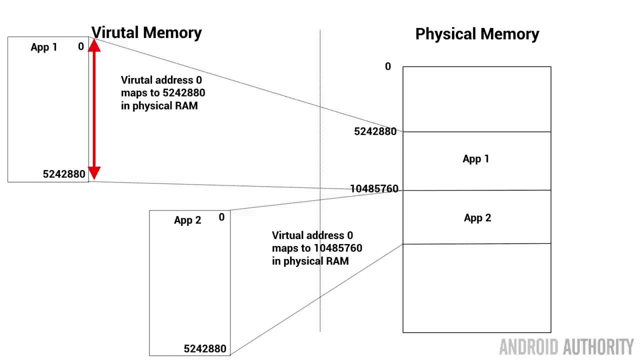 app one has an address space from zero through to 5242880.. That's about five gigabytes of memory. And I've also got app two with the same amount of five megabytes of memory And what you actually see is that, although it's from zero to there in the physical memory, 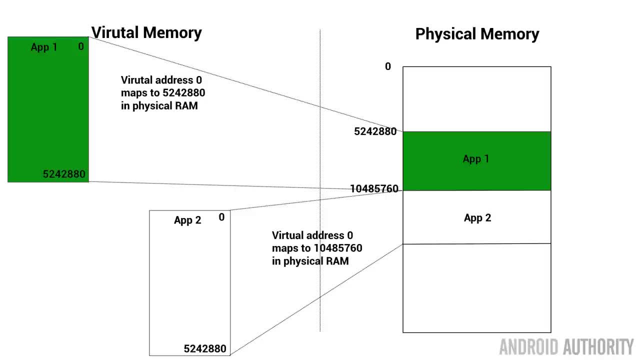 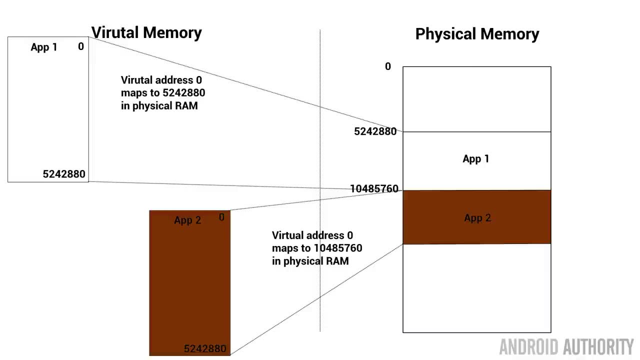 it might actually start at 5242880 and it might run for five megabytes. And then app number two actually starts at 10485760 and it runs from there for five megabytes, And the virtual address zero in both apps is actually mapped to different places in the physical. 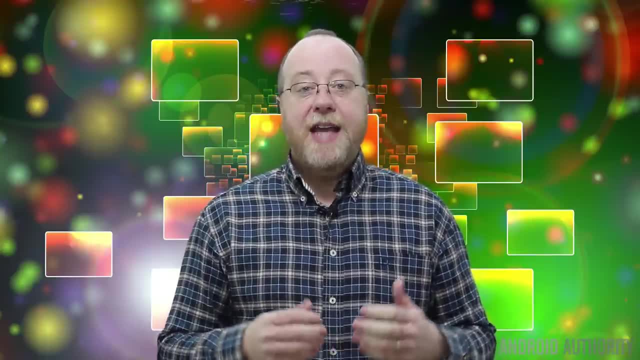 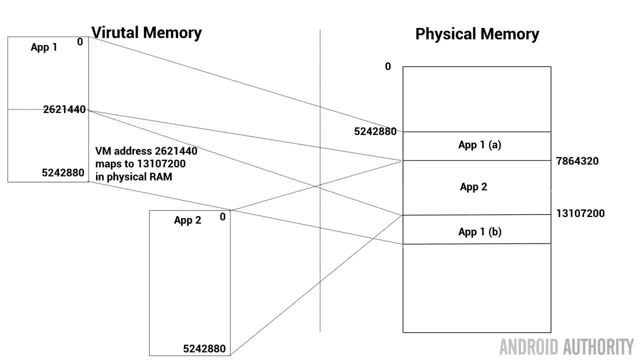 RAM. Now, because there's mapping going on here. the apps can be mapped to absolutely anywhere that the operating system wants to put them. So let's have a look at this diagram. So, as you can see here, app two is as it was before, So it's got the same number of digits. but 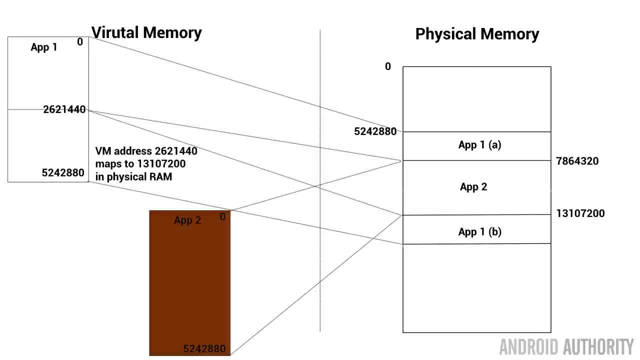 it's a five megabyte program, from zero to 5242880. And it's been mapped over to an address in the middle there of physical RAM. But app number one has actually been divided into two parts And the first half of it is mapped into memory before app number one And the 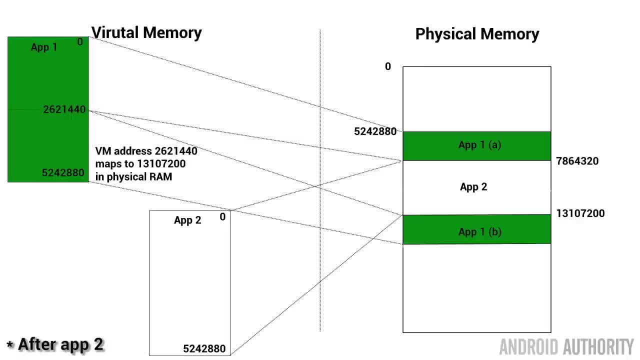 second part of it is mapped into some memory after app one. But app one and app two don't know anything about this. They just think they're running in their address space from zero to the end of their program. So you can see that the app number one and app two have. 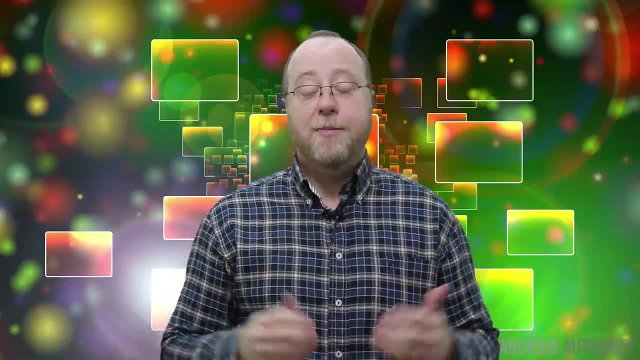 been mapped into memory after app one And the second half of it is mapped into some memory before app number two. So you can see that the app number one and app two have been mapped into their program. So the advantage of the virtual memory system: each app is self contained. It doesn't write over other apps memory space because it has its own virtual address space. Secondly, it doesn't matter where the app is in memory, because it is the MMU that does the mapping between those virtual addresses and the physical addresses. And thirdly, the. app doesn't need to be in one continuous block in memory. it can be split up over many, many different parts, And this is the OS, along with the MMU, that makes sure that each address arrives at the right place in physical ram and therefore you get rid of that memory fragmentation. 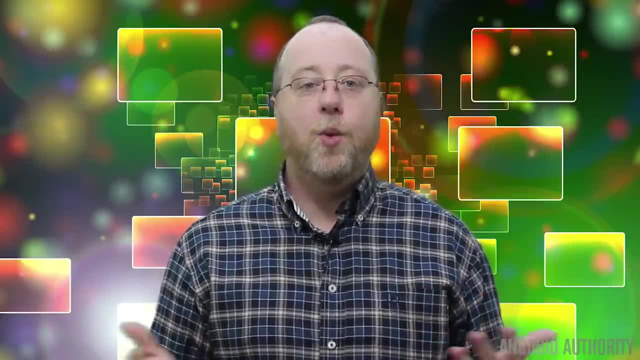 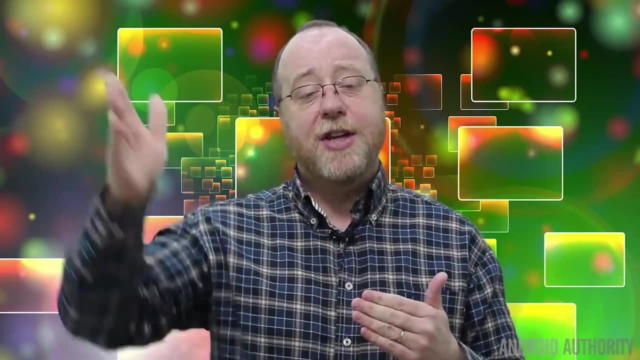 problem now. what i've shown you up until now is a one-to-one mapping, so that every time you have one particular address there's a kind of a table that gets looked up by the mmu and it tells it where to put it in physical ram. but the problem is even for a 300 megabyte program, which really 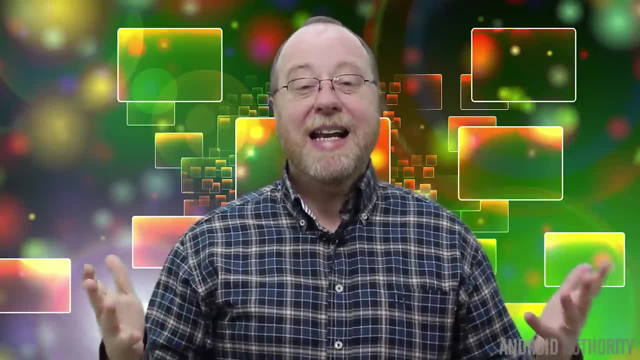 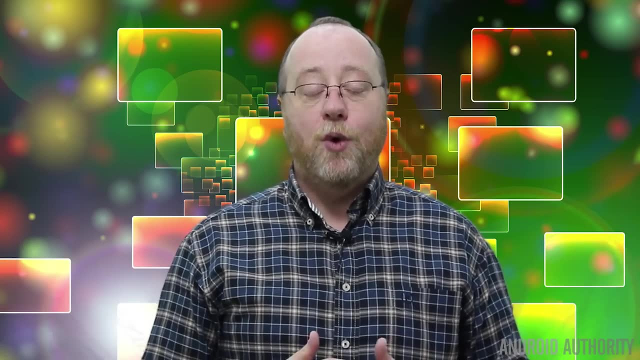 isn't that very big. you'll need about 79 million entries in such a lookup table to do such mapping and obviously if you then got 10, 20, 30, 40 different programs running on your system, that's going to quickly turn into a huge amount of data and there'll actually be no space left. 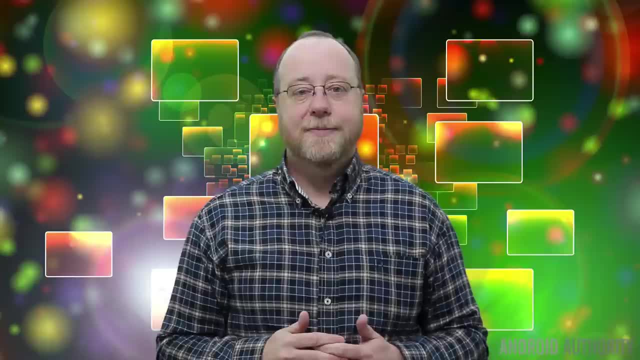 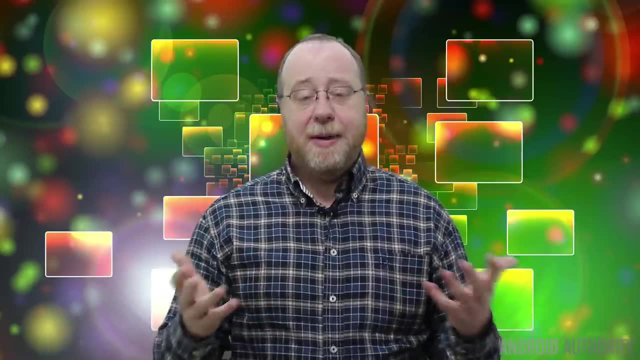 for actual programs, because it'll all just be mapping information. so to get around this, the main memory, the physical memory, is divided into different blocks and they're called pages and typically they're about 4k in size, and so now, using paging, actually you'll find that a 300. 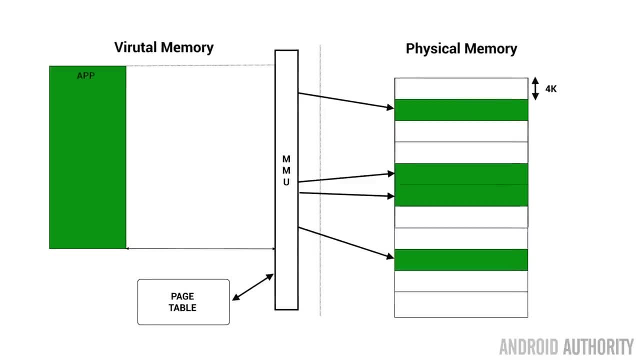 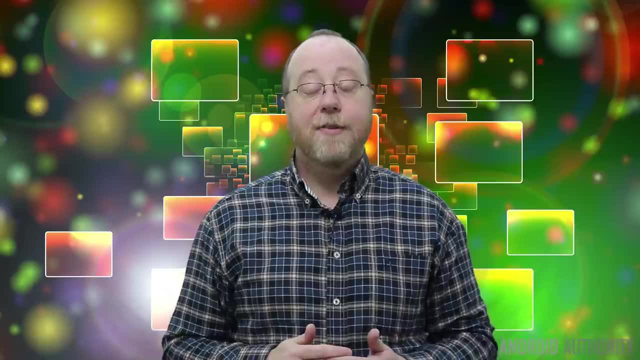 megabyte app only needs 77 000 entries in a lookup table which, at four bytes for every entry, is about 300k, which is much more manageable. so now what happens when an app requests something with a virtual address? it actually goes to the mmu. 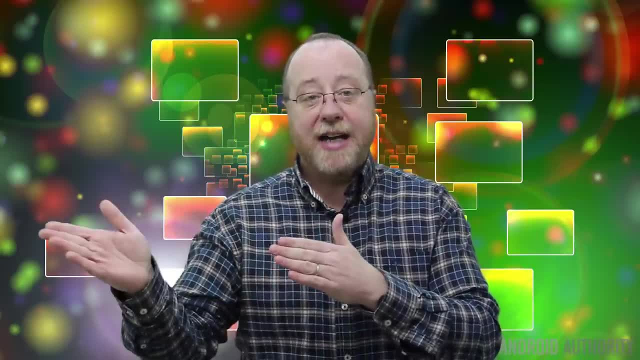 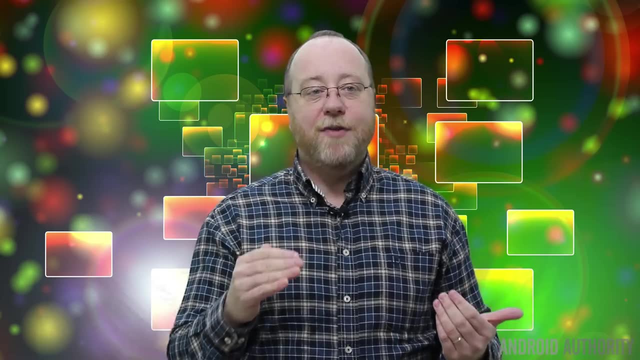 and the mmu finds out which page it's in and redirects it to the physical address of that particular page. however, what happens when the address is in the middle of a page? the start of the page is easy. there's a kind of a one-to-one lookup. but what happens if it's in the middle of? 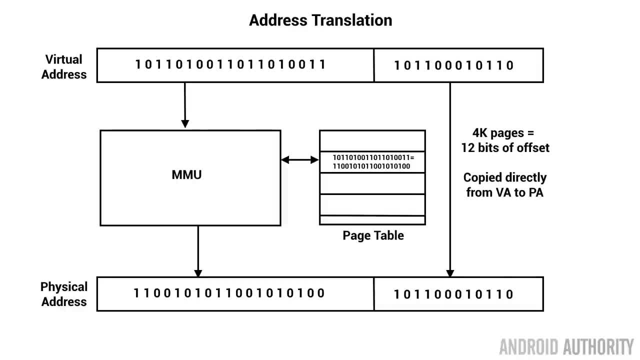 the page. well, actually what happens is that four k is 12 bits. so the first 12 bits of the address are copied directly from the virtual address into the physical address. then the remaining 20 bits are used as the page lookup. that 20-bit address is looked up in the page table. a thing called a page table entry is found. 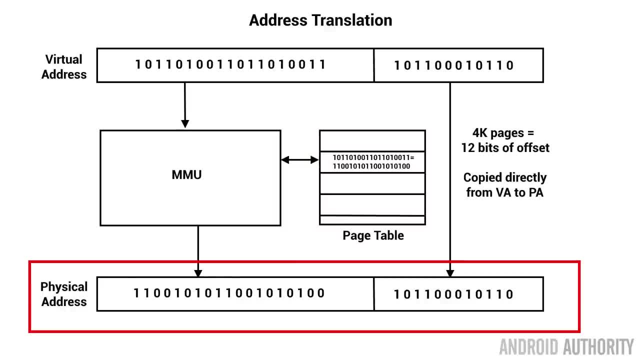 and that then gives you the 20 bits for the upper part of the address, and then the combination of the page address and the offset, those 12 bits gives you an actual physical address in ram. now one interesting question is: where are all these tables held? well, they're not held in the 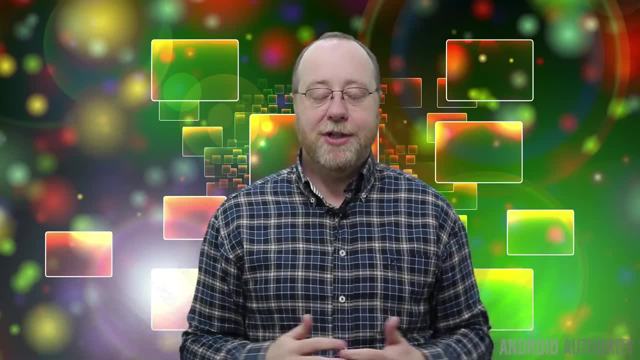 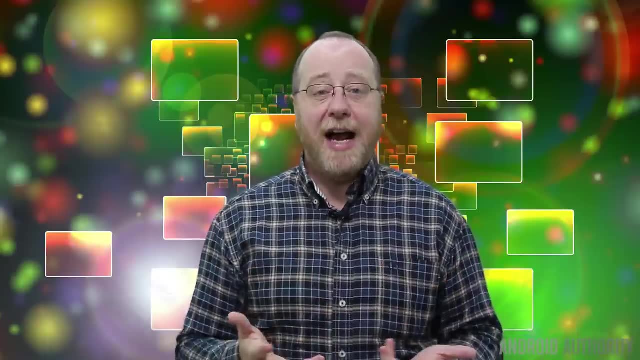 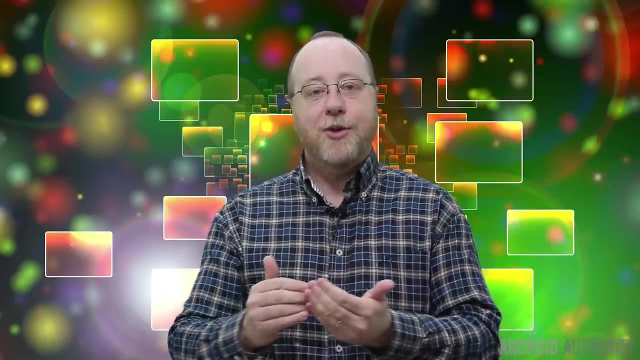 cpu, because even at 300k or 400k, multiply that by many, many, many processes running, there's just not enough space in a cpu to do that, so they have to be held in ram. now that leads us to a kind of an interesting conundrum, because to access a virtual address, the mmu needs to access physical ram. 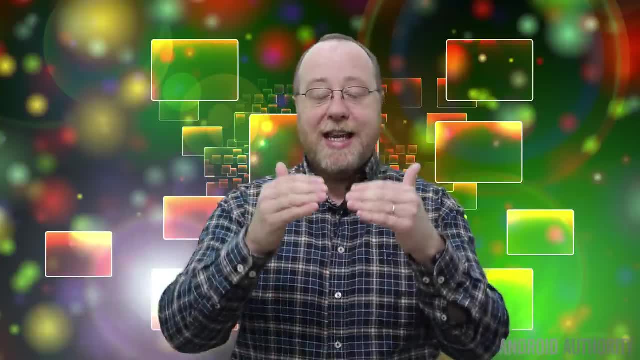 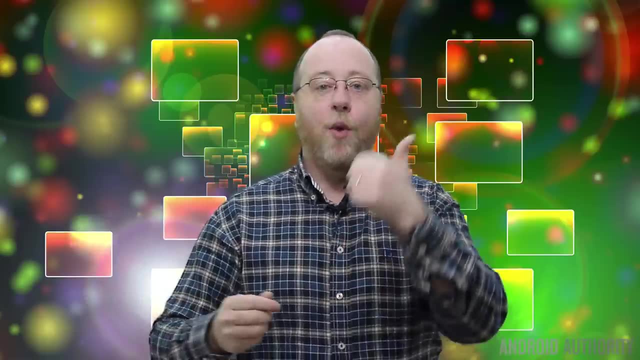 to find an entry in the table so it can then translate the virtual address into a physical and then access ram again. so you find there's multiple ram accesses happening for one ram access inside of the app and of course that's going to be slow if it's like two ram access is needed, or 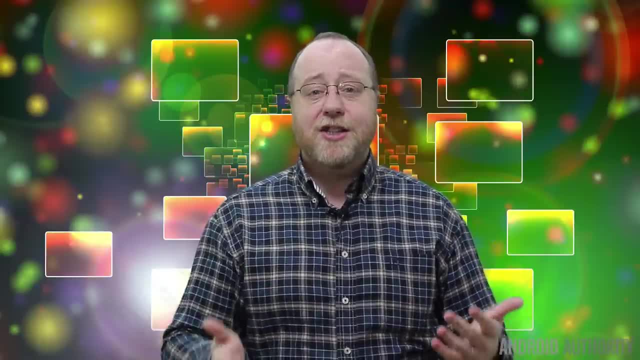 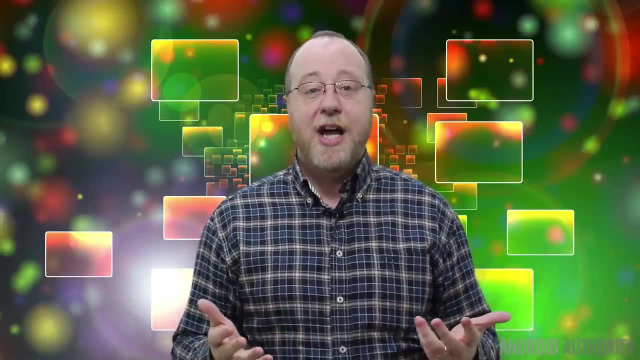 three ram access is needed for each uh virtual address and that's going to slow down your program by by a factor of three. so the way cpu designers get around this, they have a cache, a cache of recently looked up addresses. it's actually called the translation. look aside. buffer the tlb. 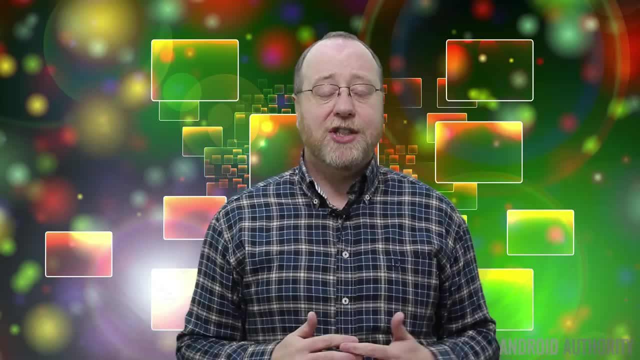 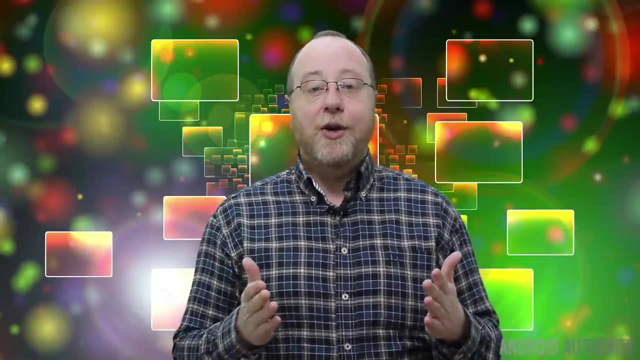 and what that does is whenever there's address translated, it gets stuck into this cache and then the next time an address is needed, actually it looks it up in the tlb, but of course, remember, it only needs to look up the page size. so if the program is running through the different instructions, 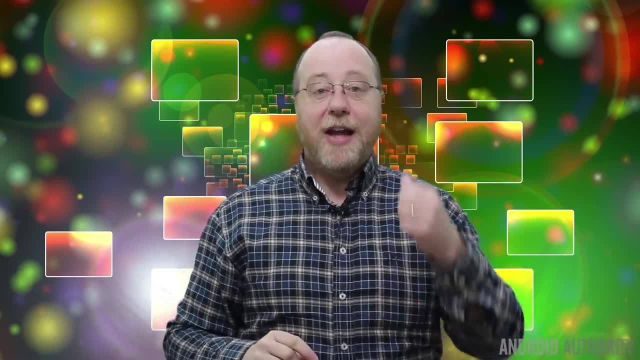 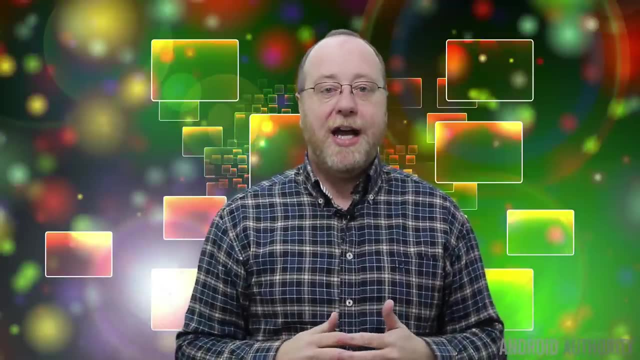 inside of one page. every time it goes to access it, it will automatically be a tlb hit, because that page has already been found and just the offset changes, which is absolutely okay. in some cpus, in fact, the tlb is only 20 entries long. it might be bigger than that. 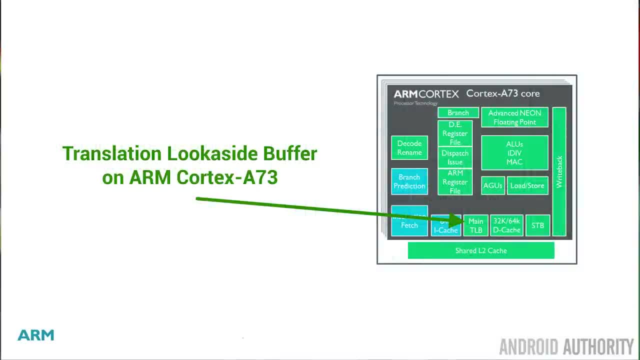 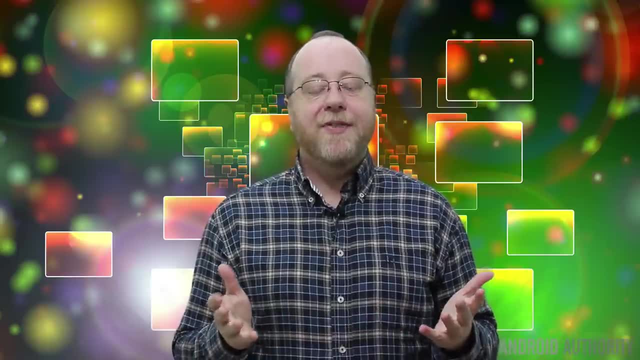 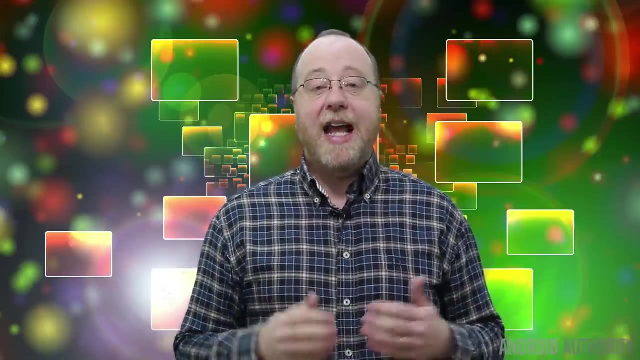 maybe 64, 128, but you don't need that many tlb entries to actually increase the performance significantly during this lookup. so what happens if the mmu can't find an entry in its table for a particular virtual address? well, in that case the mmu raises a page fault. 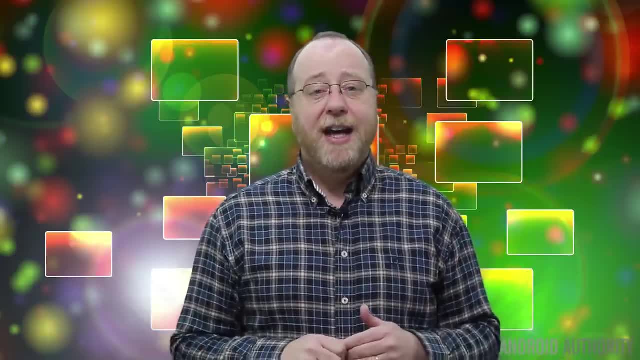 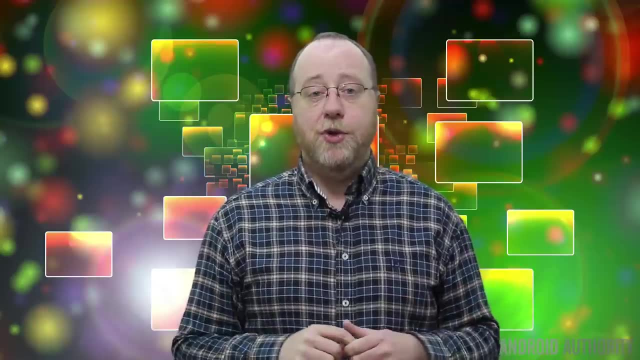 and it goes back to the kernel saying, hey, i can't find that address now. that can happen for one of three reasons. first of all, the app is actually trying to access an address which is not allowed to access. it hasn't been allocated that memory and therefore linux will just basically. 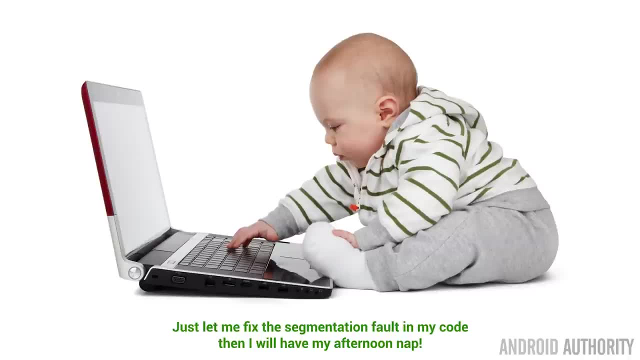 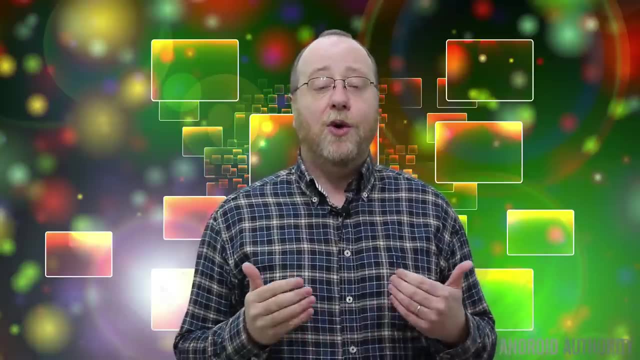 kill it off, you get a segmentation fault and the program just crashes and just it just gets wiped out of memory because it's not allowed to access memory that it hasn't been given. in the second case, it could actually be what they call lazy allocation, which means that the kernel said yes. 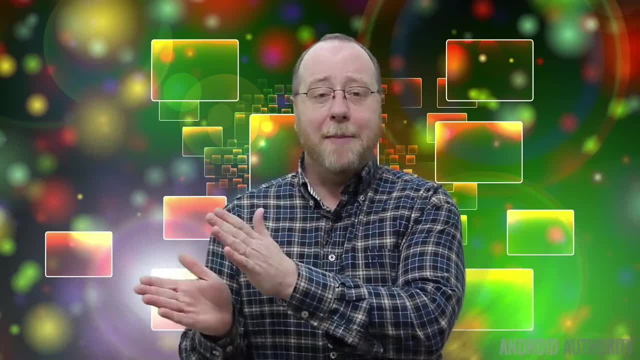 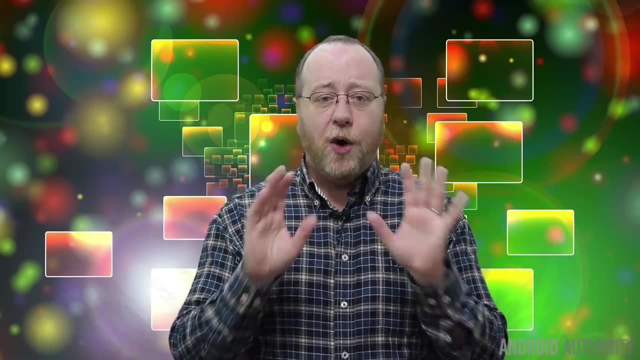 you can have that, but it won't actually give it a physical page of ram until it actually starts to write to it, and so in that case the page fault happens, the kernel says it's okay. and the kernel says okay, i told the app it could use that memory. here is where i want you to put it in physical ram. 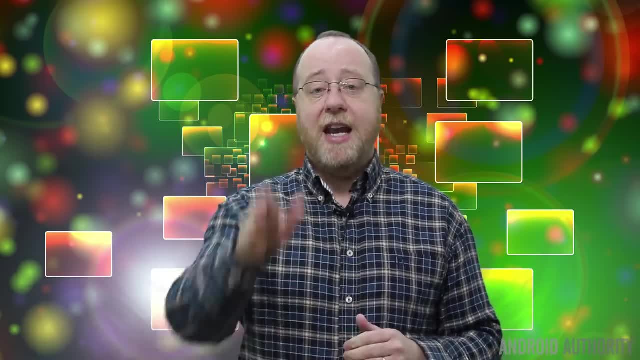 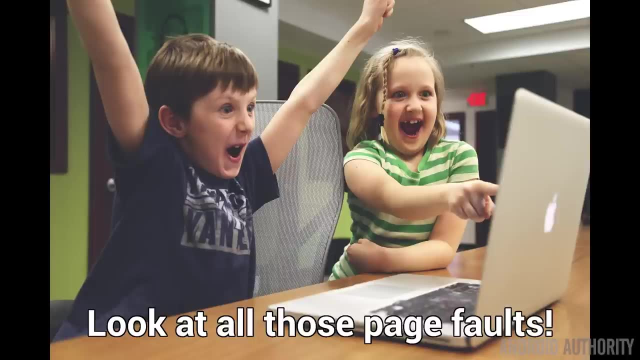 the mmu is reprogrammed and then the whole thing starts off again and the address is found in physical ram. and the third thing that can happen is the mmu says we used to have that memory but actually now it's been swapped and therefore the kernel will go and get that page from the